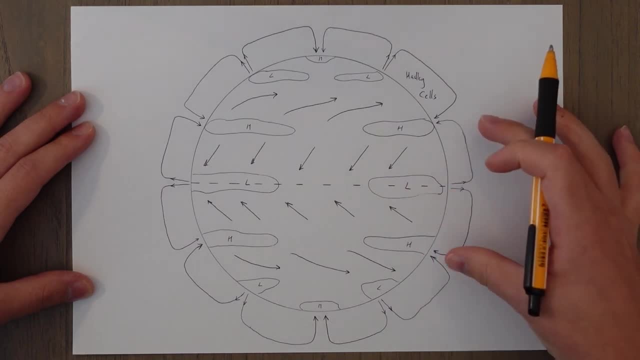 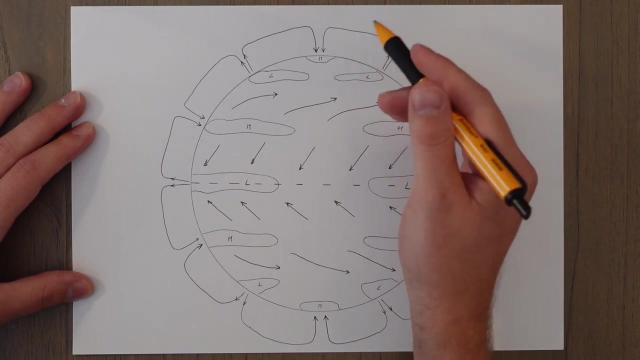 the tropopause spreads out, cools down and starts to descend in the subtropical regions, leading to high pressure. the inverse of this is true at the poles: the surface cooling, the very cold temperatures of the poles create areas of high pressure that pull down the air and it sucks in air from the mid latitudes say. we end up with three Hadley. 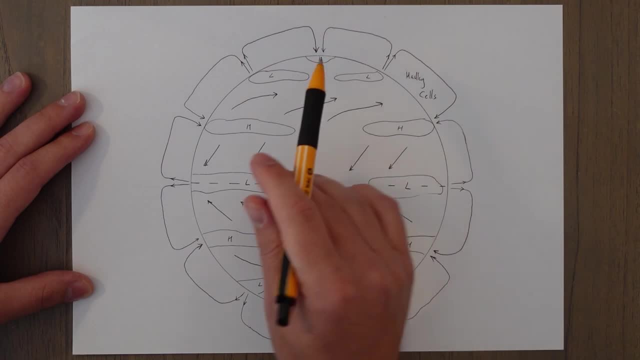 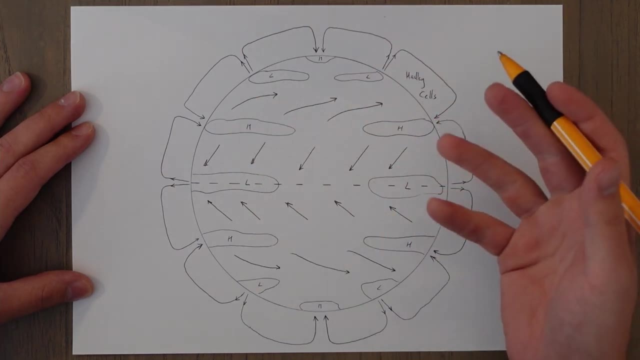 cells in north and three Hadley cells in the southern hemisphere. this is obviously a cut through view. in reality, they would be um like doughnut shape. these Hadley cells drive the various weather conditions year round or climates such as sunny, hot deserts and stormy equatorial. 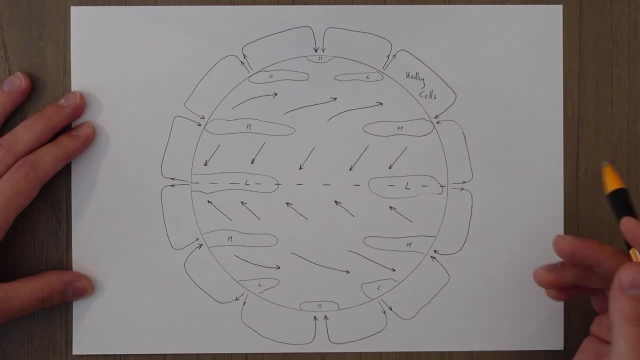 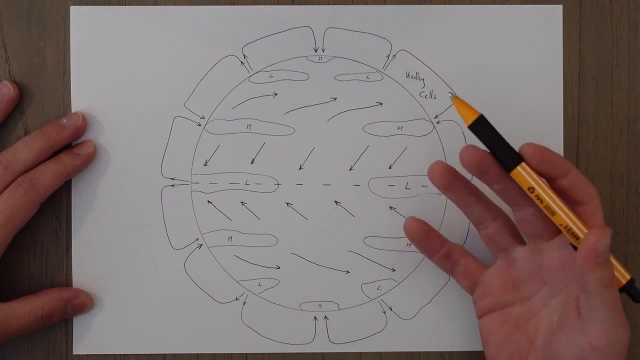 regions which we're going to have a talk about just after we've covered. the winds here air for flows from high pressure to low pressure and then it feels the effects of the geostrophic or coriolis force. this means that we have some winds that are fairly consistent year round. 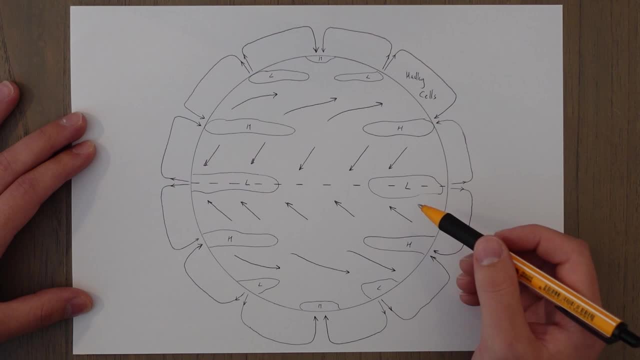 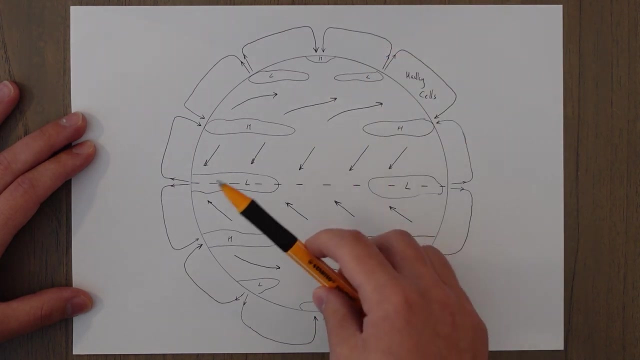 if we look at the equatorial region, we see air flowing towards the equator from the subtropical highs. the coriolis force then pulls it around to the right in the northern hemisphere and in the southern hemisphere it pulls around to this left. this means that in the northern hemisphere around the equator, we get north easterly winds. 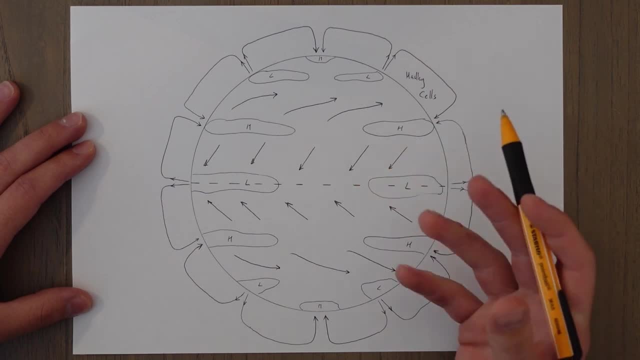 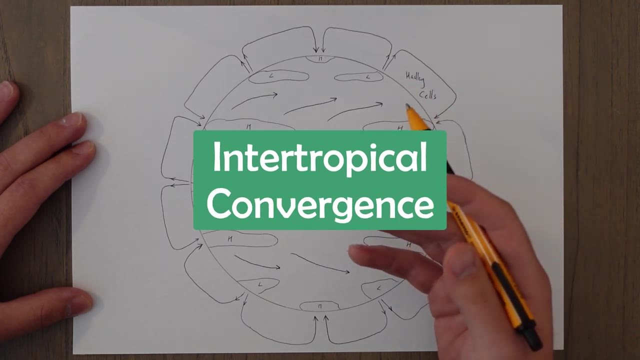 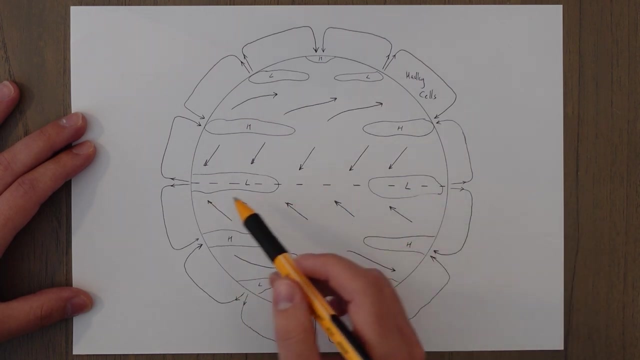 and in the southern hemisphere we get south easterly winds, which are known as the trade winds. where these winds meet, we call it the intertropical convergence zone, the itcz, and the position of this intertropical convergence zone will not always be directly along the equator. 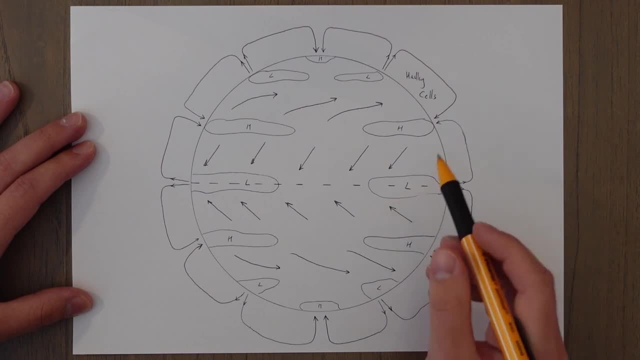 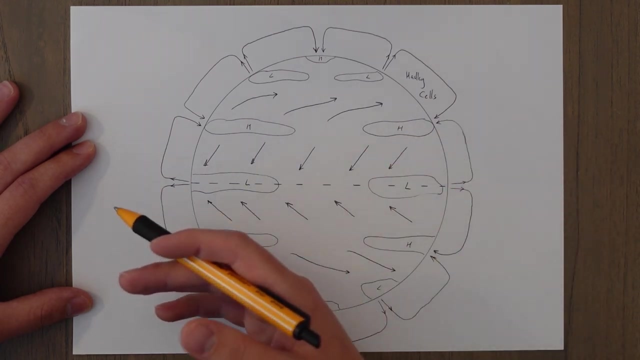 this is because the equatorial lows that are driving this whole system won't always be directly along the equator either. they will move north in may to august due to the northern hemisphere summer, and move south in november to february during the southern hemisphere summer. this means that the line of the intertropical convergence zone and the resulting trade wind convergence will also move north and south with the seasons. we'll also see fluctuations due to the difference of heating on the land versus water. land heats up and cools down better, so we see large rises. in temperature over the land in the summer and basically in the southern hemisphere there's a lot less land than in the northern hemisphere, so we see the intertropical convergence zone fluctuate a lot more when it actually hits the land compared to when it's over. 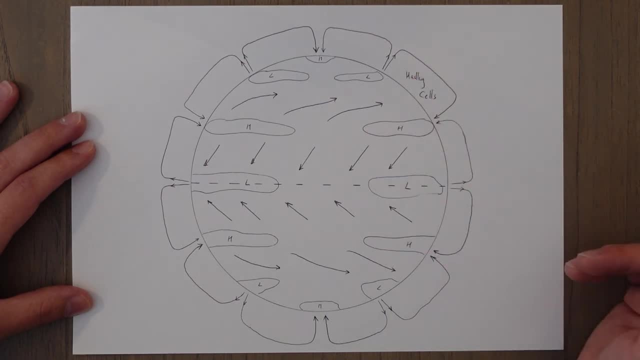 the sea, and that means that the trade winds move as a result of this. so, other than the trade lens in the mid latitudes, we see air masses moving from the subtropical high towards the mid latitude low pressure areas and again the coriolis force is uh acting on these air masses and it pulls it around. 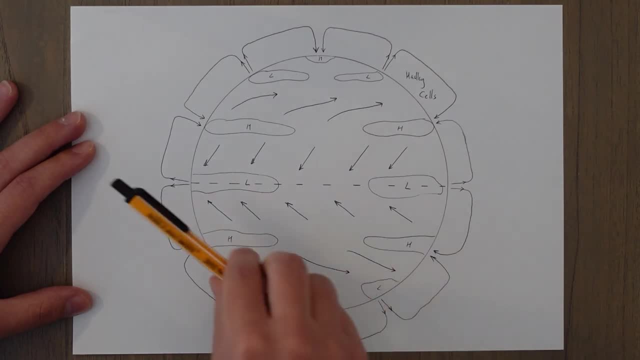 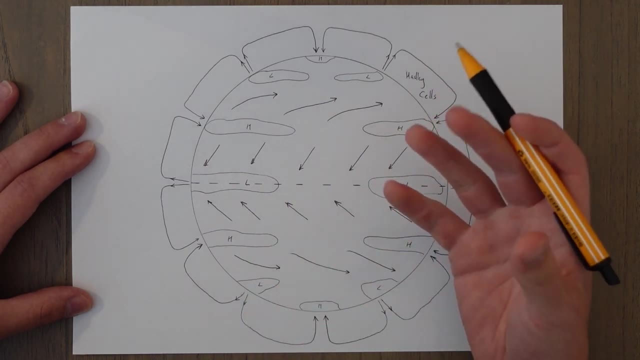 to the right in the northern hemisphere and then it's high to low in the southern hemisphere and it pulls around to the left, so we get generally westerly direction winds in the mid latitudes. yeah, wind blowing over the Atlantic and blowing over the Indian Ocean In the Southern Hemisphere. 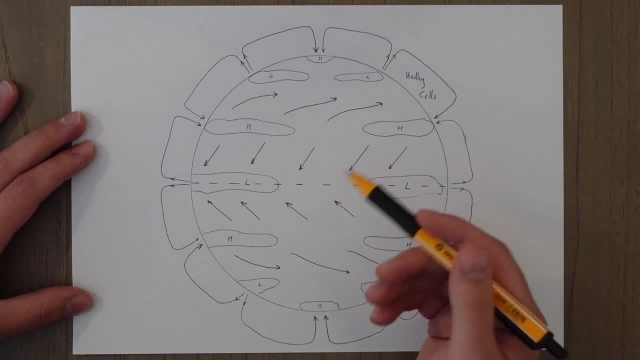 especially, these can get up to very fast speeds. again, because of that lack of land in the Southern Hemisphere, it means that there's nothing to create too much surface friction and these can quickly carried away, which is why sailing in the Southern Ocean around Antarctica is renowned for. 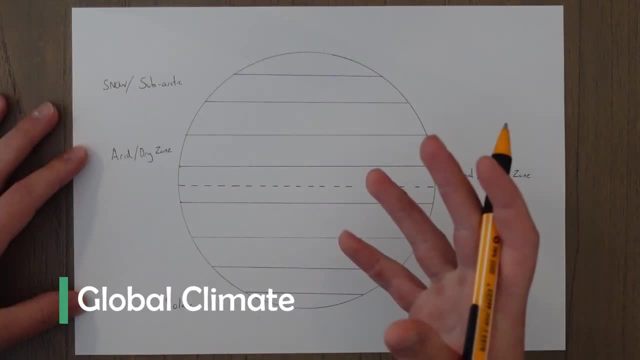 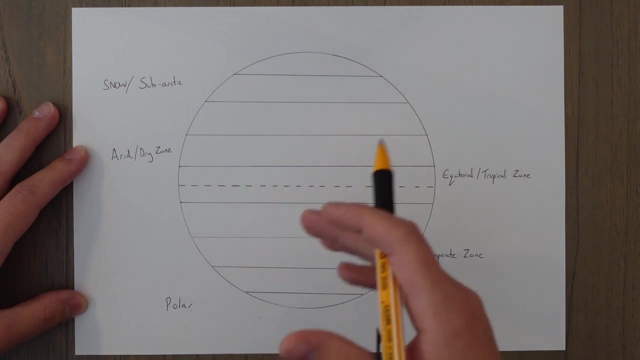 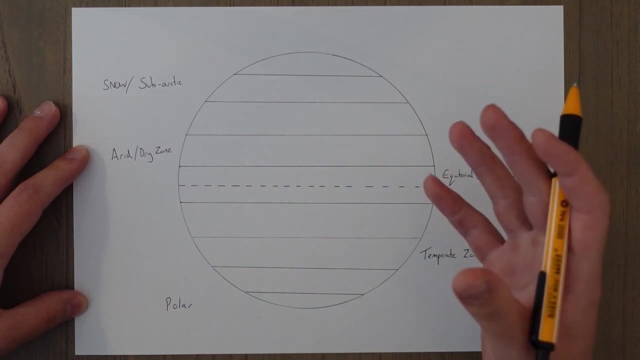 being very difficult because of these high winds. Defining climates is quite a difficult thing to do because there's a lot of nuance, detail and local factors that can be involved in a specific climate for a specific area. but there are quite a lot of different climates and one of the easiest ways to 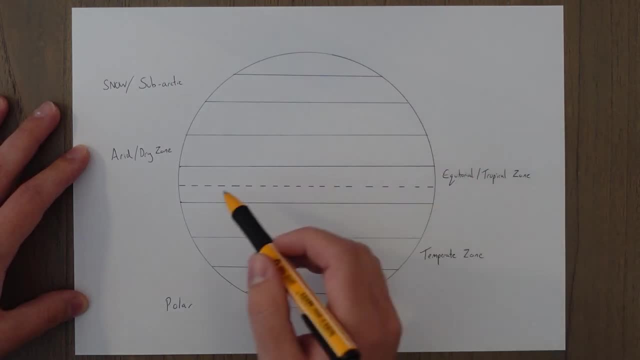 break them down is based off of latitude, So the first one we're going to start with is the equatorial zone or the tropical zone. It can also be split down into rainforest and savannah, So the rainforest is the equatorial zone and the tropical zone is the equatorial zone, So the rainforest is the. 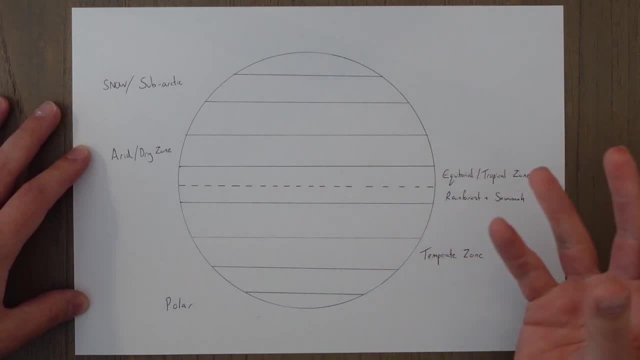 closest to the equator and we see very little in the way of any seasonal variation. We see the low pressure areas caused by these Hadley cells, which means we get high levels of convective weather and high levels of precipitation and storms year round. If we move slightly further away from the 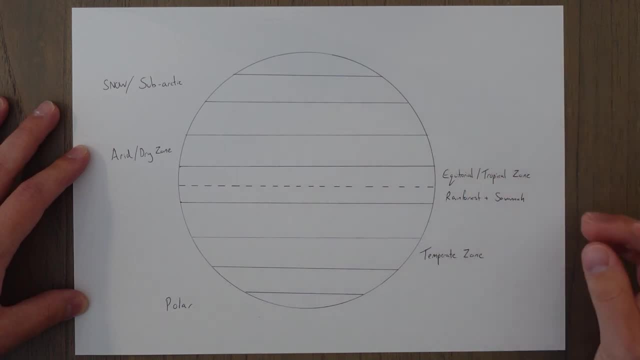 equator. it's a little bit cooler than the rainforest just because it's a little bit further away from the equator and it results in a little bit more of a seasonal variation and we get distinct dry and wet weather. So the rainforest is the equatorial zone and we see very little in the way of any seasonal variation. 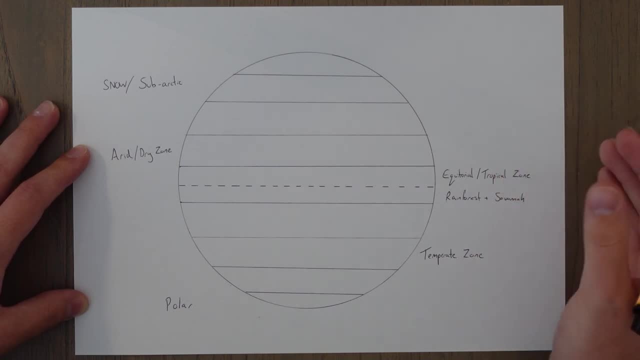 So the rainforest is the equatorial zone and we see very little in the way of any seasonal variation. We see wet seasons again, with quite convective weather. so you see storms coming to the savannah when it's the wet season and in the dry season not that many storms and, yeah, animals struggle to find water. 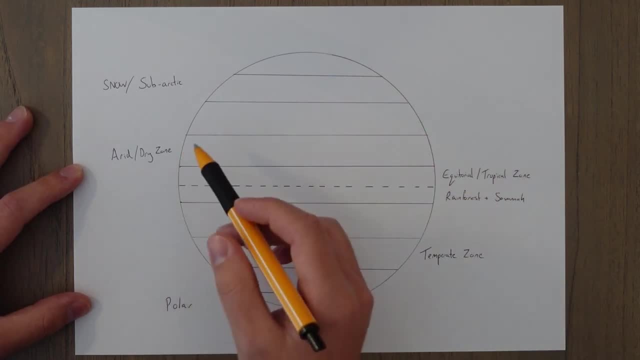 and things like that. Next, furthest away from the equator, you would get the arid or the dry zone. This can be in the form of either a desert or a steppe region. Basically, what happens is these Hadley cells are pushing down, causing a very low level of rising air, and that can be a very low. 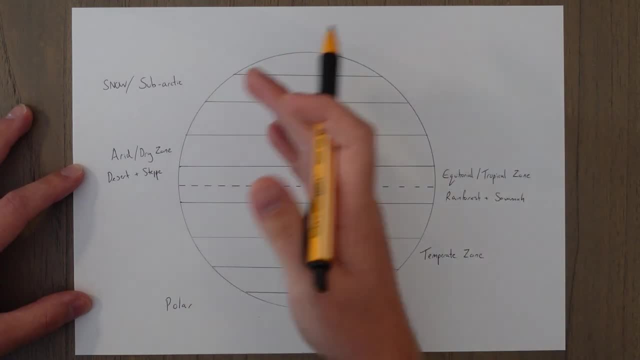 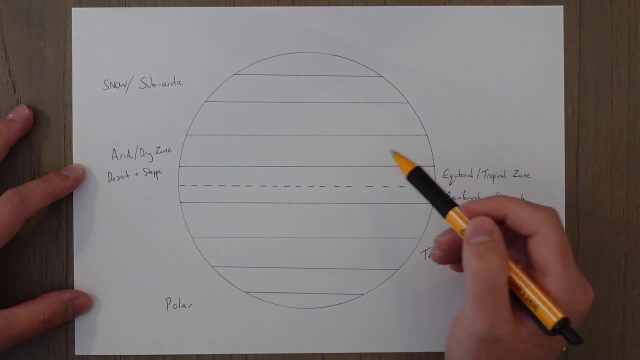 air and rising moisture. because of that low level of rising air and rising moisture the sun is able to penetrate and hit the surface of the earth, make it very hot, make it very dry. but in the step regions you are a bit further away from the equator, so you do get a slight bit more precipitation. 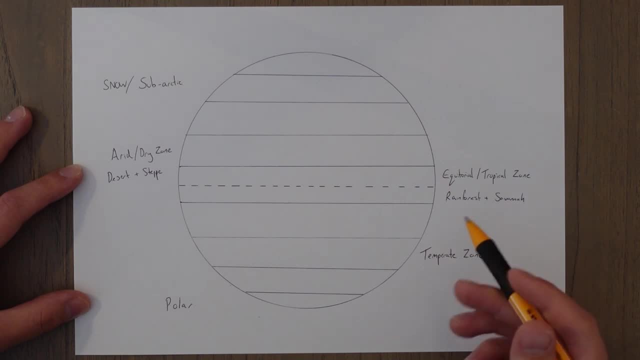 and rain as a result. Next out you get the temperate zone, which is where the majority of the world's population live, and it can be either cool or warm, which is sometimes referred to as mediterranean. In the cool temperate zone we see quite high seasonal variation, with lots of 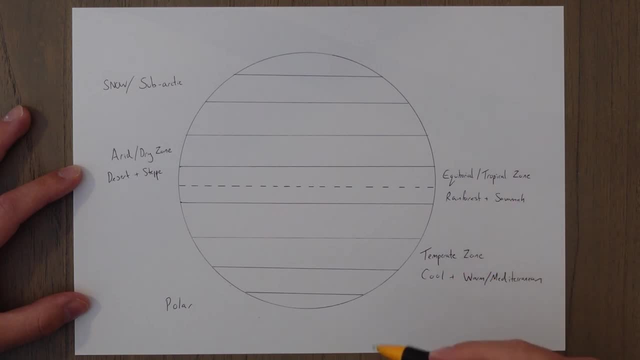 precipitation year round and we get the four distinct seasons of spring, summer, autumn and winter. In the mediterranean or the warm temperate zone there is still high seasonal variation, but it's not to the same extreme levels as in the cool temperate zone and we often get 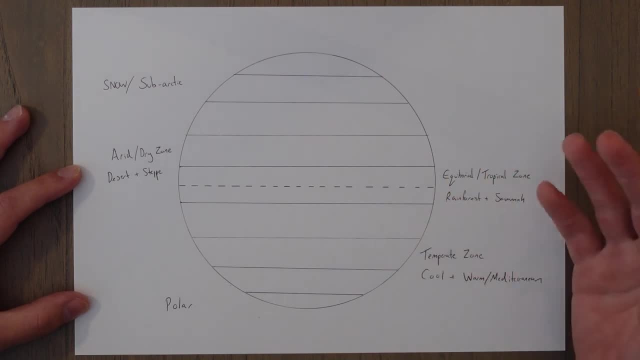 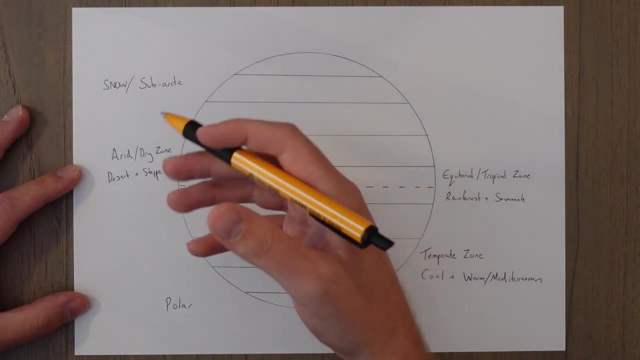 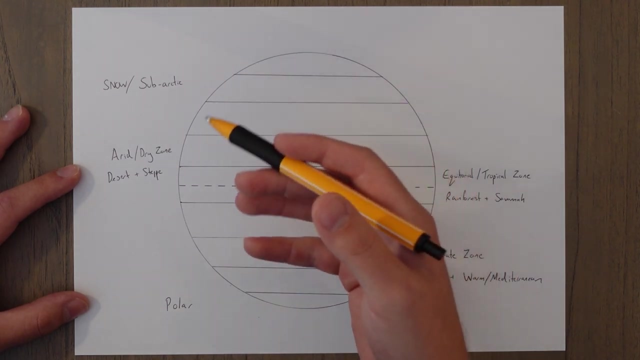 hot, dry summers and warm, wet winters. Next, furthest away, we get the snow or the sub-arctic region, and it's where we have a large seasonal variation, predominantly down to the large surface heating effects caused by the large areas of land, predominantly Russia and Canada. There's a 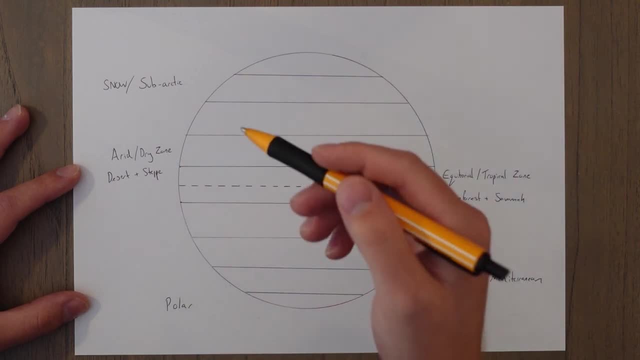 lot of land there, a lot of land to get hot, a lot of land to get cold. so we see very hot summers and also very cold winters, and they last a very long time. After that, you get the polar region, the polar zones, and this is where we get very extreme seasonal variations, featuring incredibly 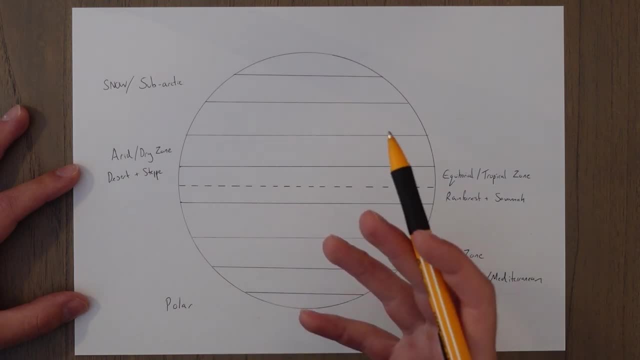 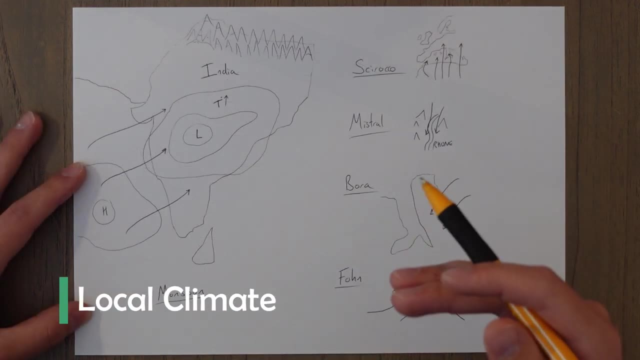 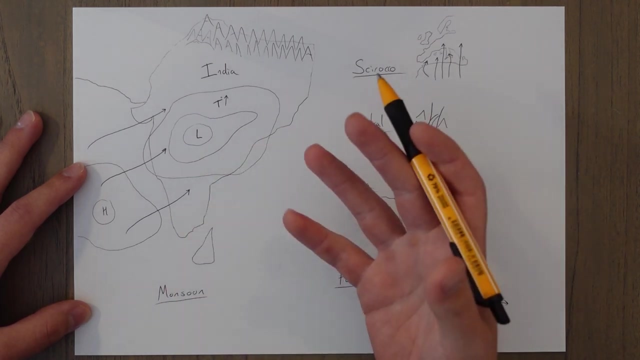 cold winters. We also get constant daylight in the summer and constant night during the peak winter, because we are in the arctic circle. So within the large climate latitude zones there are factors that will affect the local weather which can vary from day to day, such as pressure patterns. 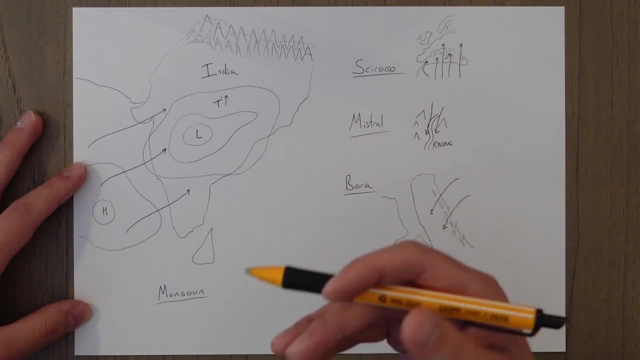 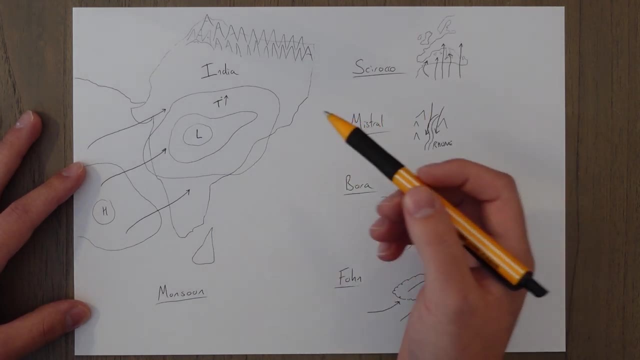 fronts, moisture levels, etc. There's also some more long-term, month-to-month factors which can have an effect on the local climate as well. One of the main ones is called the monsoon which is experienced in India, for example. Basically, what happens is there's different levels. 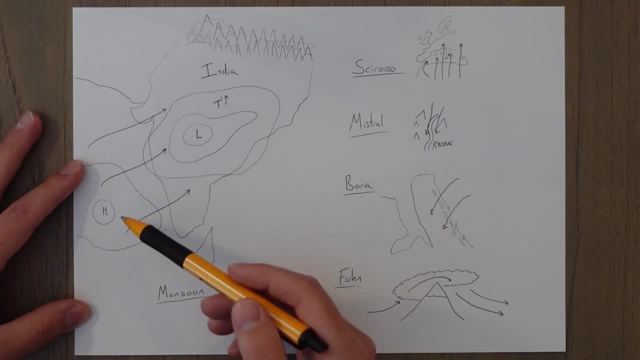 of surface heating in the summer between the land and the ocean. This causes a large low pressure area on land when compared to the ocean and a large flow of air inland. It's essentially a large-scale sea breeze. It brings with it a lot of moisture-filled air and heavy precipitation storms. as it does this. 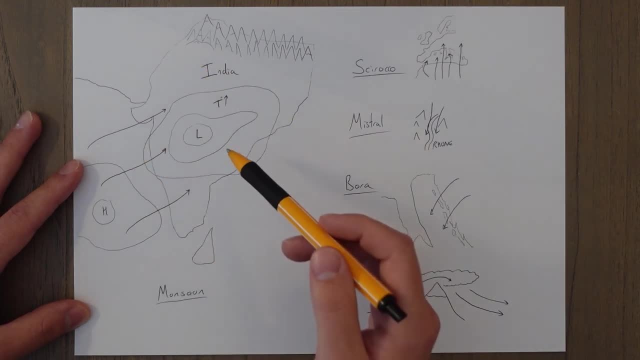 In the winter the process is reversed and the land cools down more than the ocean. it has a higher pressure and we see your air flowing out into the Indian Ocean with very little water because it's been over land. it's nice and dry. Monsoon climate is primarily associated. 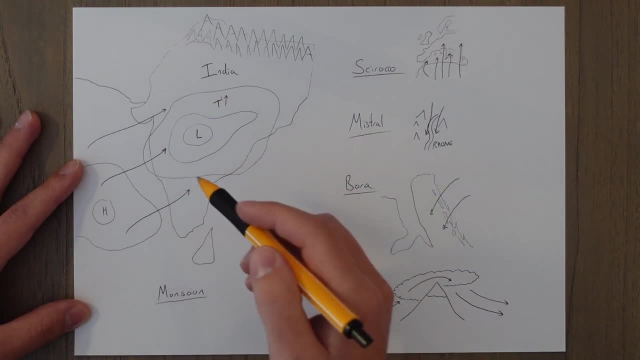 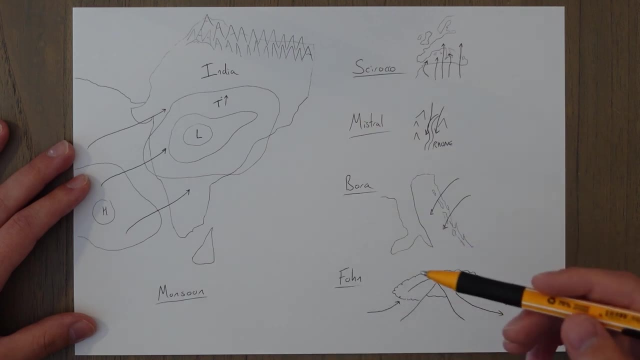 with India, but it's not exclusive to India. They're also experienced by North Australia, West Africa and Australia. So mountain chains or other topographical features may affect the weather and produce seasonal wind patterns that can affect the local climate for a period of the year. 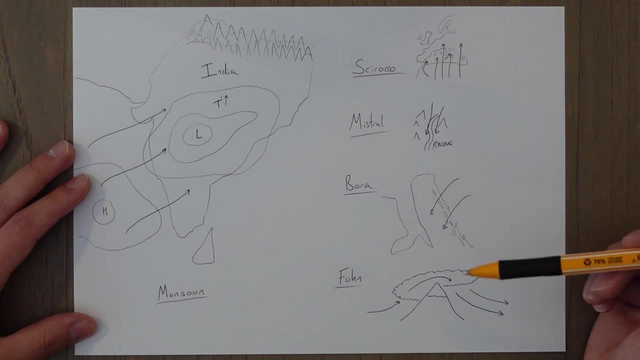 There will be some specific ones for wherever you live, but some common ones that are experienced in Europe. where I live, are the Chiroco Wind, which is a hot, dry and dusty wind which blows north from the Sahara. You get the Mistral Wind, which is a northerly breeze which blows down the Rhone Valley. 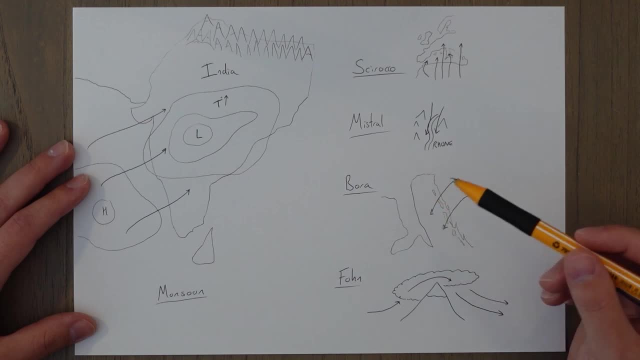 You get the Bora Wind, which is a katabatic wind flowing down over the mountains in the Balkans towards the Mediterranean, and you get a lot of Fone Winds, which is a warm wind that is formed by the adiabatic warming of the air after crossing a mountain peak. So the climate is very often driven by latitude. 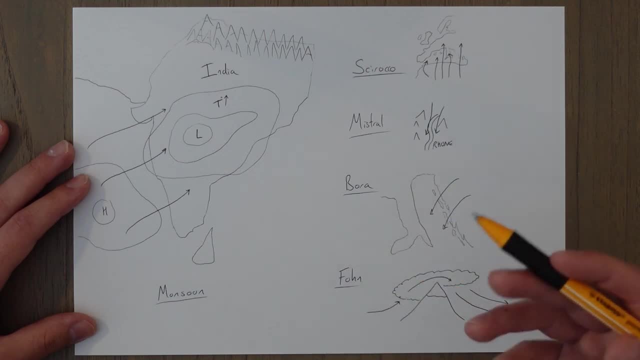 season and local factors such as mountain ranges or large masses, but the weather won't always follow the predictions that come with the climate you're in. They should generally follow that pattern for some reason. It's true for sustained periods of time, but you will see variations from day to day. 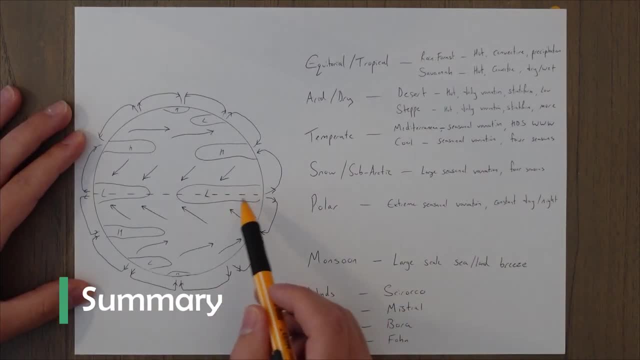 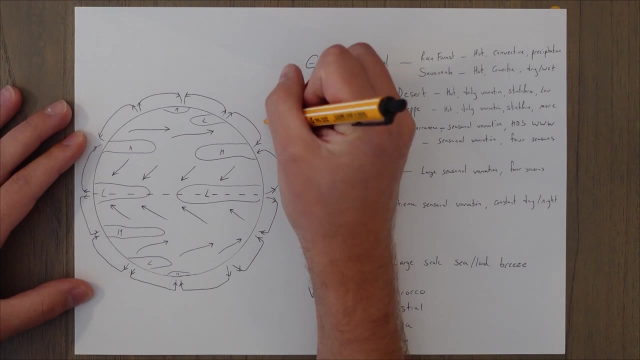 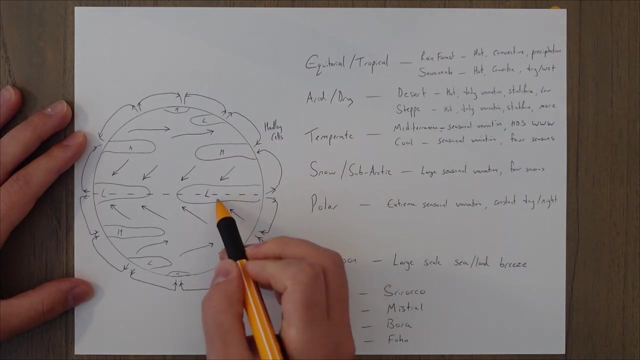 So, in summary, then you get surface heating causing low pressure. areas around the equator leads to rising air which spreads out and falls back down to the earth in what is known as Hadley Cells. These Hadley Cells produce high pressure in the subtropical regions, low pressure in the equatorial. 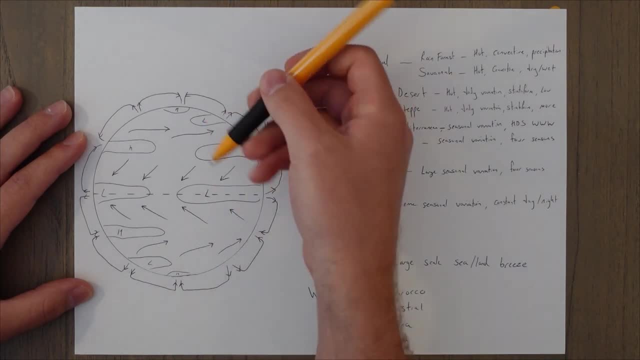 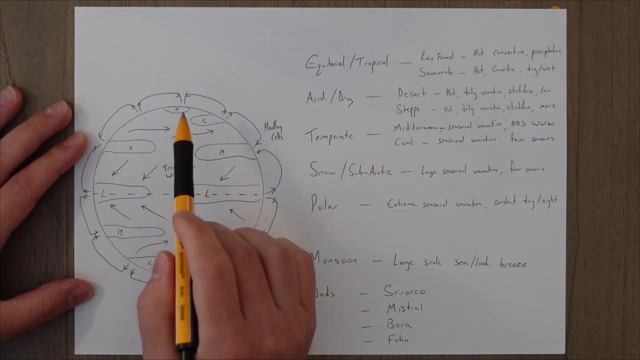 regions, air mass flows from high to low gets pulled around to the right in the northern hemisphere or to the left in the southern hemisphere, Creating the trade winds. The same thing is happening at the poles, but it's the reverse process. The poles are very cold, so they pull air down, creating high pressure, and this pulls in air. 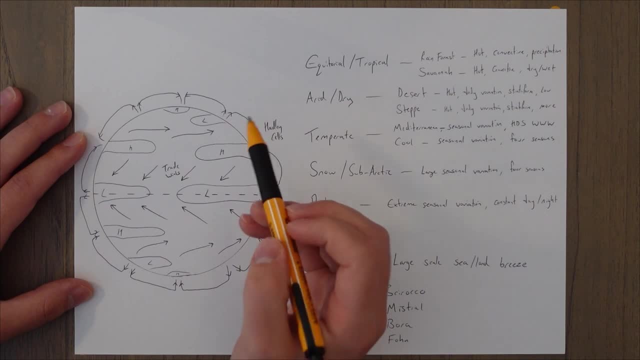 from the mid-latitudes, creating low pressure area Again. the high pressure area at the subtropical regions and the low pressure area at the mid-latitudes causes a flow of air which is then pulled around to the right in the northern hemisphere or to the north hemisphere. 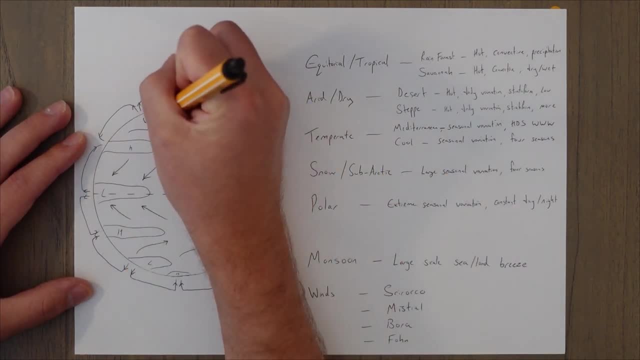 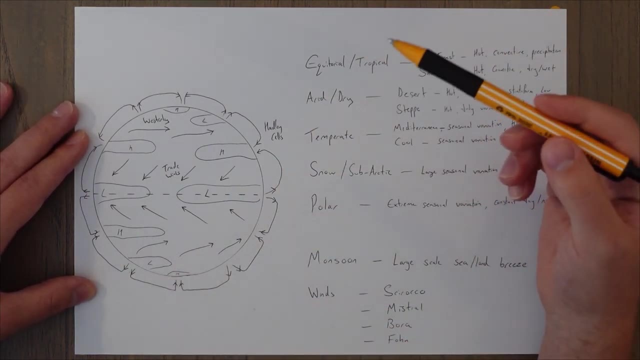 So we get general westerly winds in the mid-latitudes. The climate is based on a number of factors, but one of the main ones would be the latitude that we're at. You get equatorial, dry or arid, temperate, sub-arctic or snow and polar. 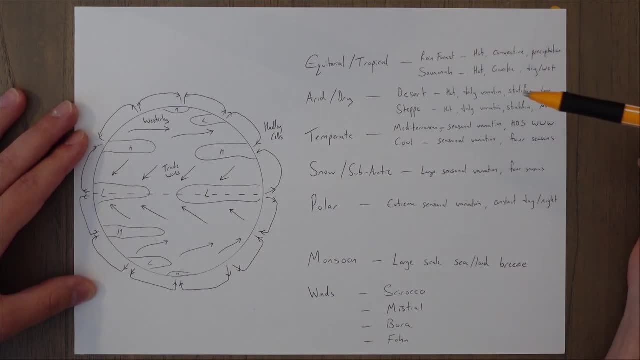 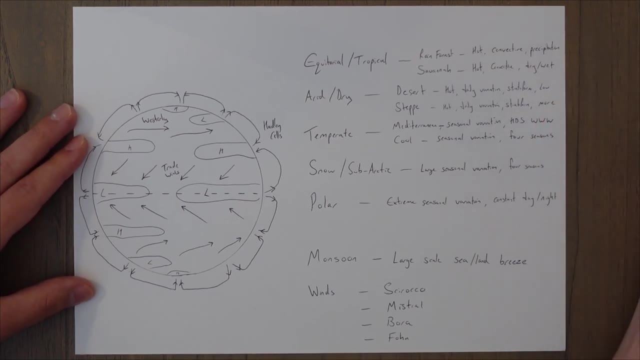 In the equatorial regions. we can break it down into rainforest, which is right by the equator. It's very hot, very convective, a lot of rain in the form of storms and, yeah, storms, really In the savannah it's a little bit further out- You still get. 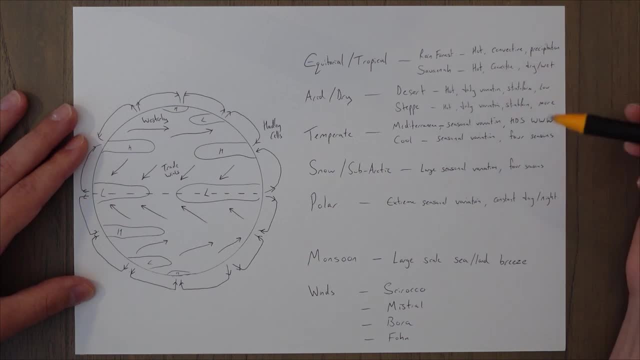 convective weather, but you get a distinct dry and wet season. In the dry regions we can break it down into desert or steppe conditions. Deserts are hot, high pressure, very high daily variation because there's not much cloud cover and it means that there's very low. 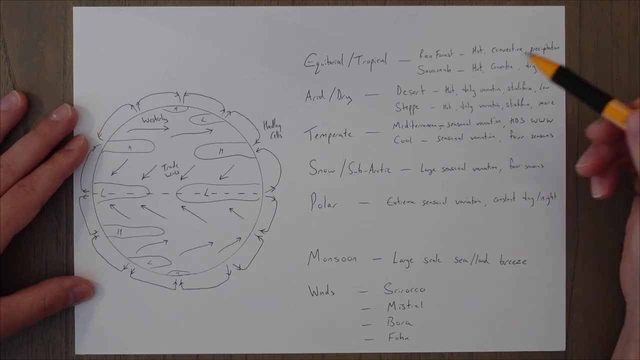 precipitation as a result, The steppe region is slightly further out. We still get high daily variation in temperature between the night and the day. There's a little bit more moisture, so we get slightly more weather and rain- sorry than the desert regions In the temperate region, where 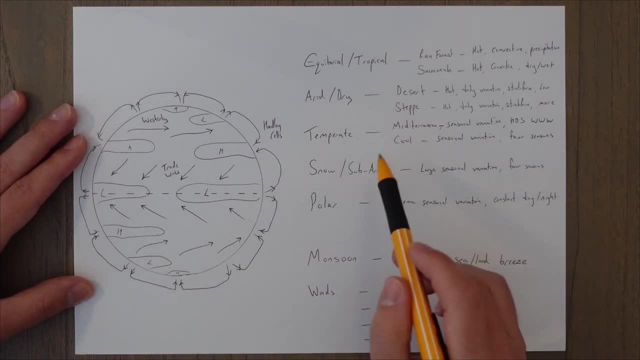 most of the world's population live. we get Mediterranean climates and cool climates. Mediterranean climates have four seasons. We get hot, dry summers, warm, wet winters and a spring and an autumn. in between, And in the temperate cool zones we get high seasonal.